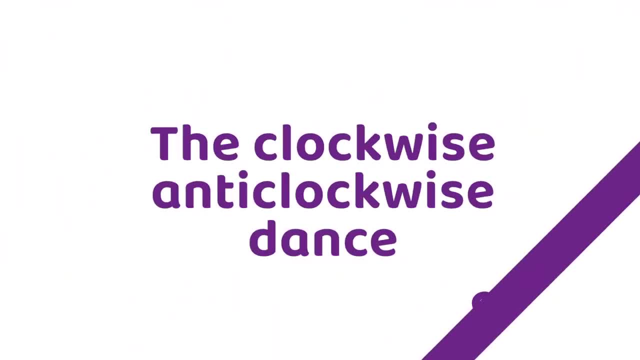 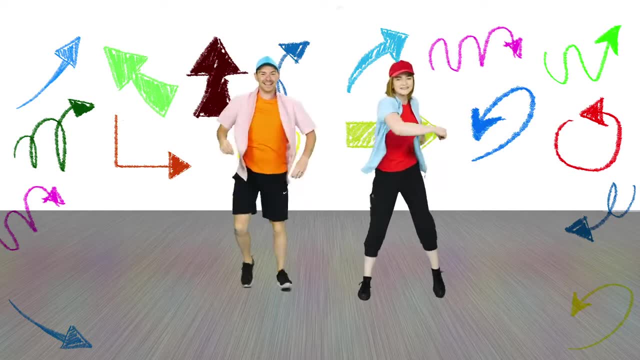 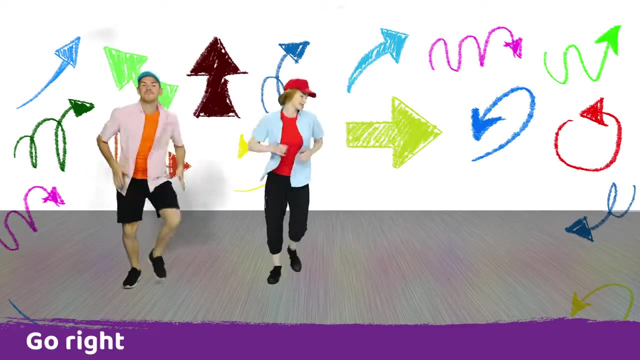 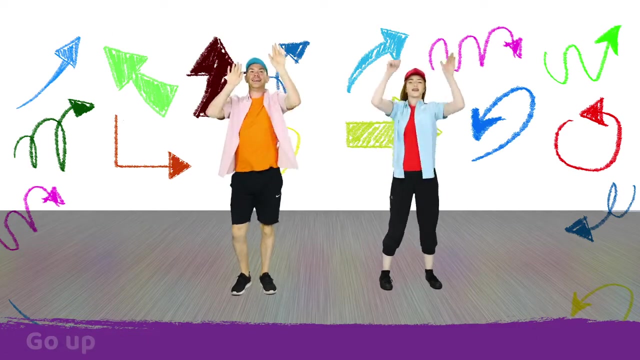 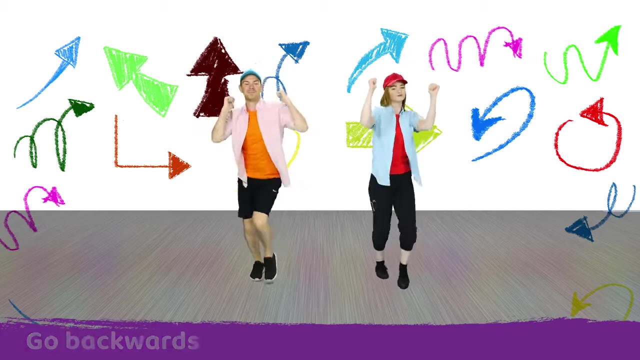 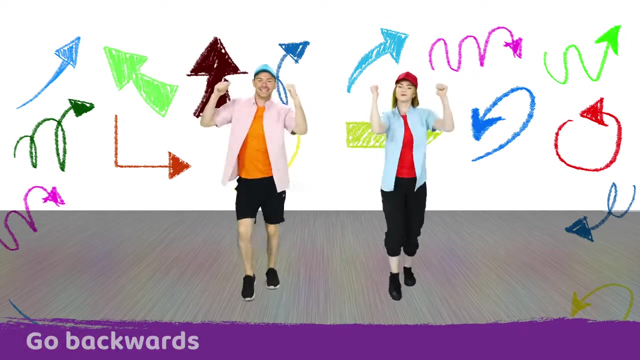 This video is sponsored by the Doctor Who logo at�. I can go backwards, I can go forwards. I can go backwards, I can go top, I can go middle, I can go bottom, and again I can go forwards. I can go backwards, I can go forwards, I can go backwards. 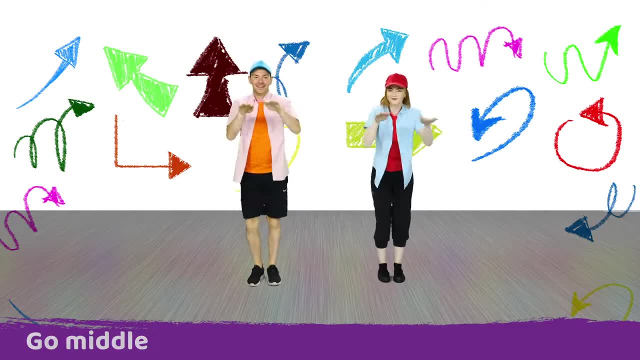 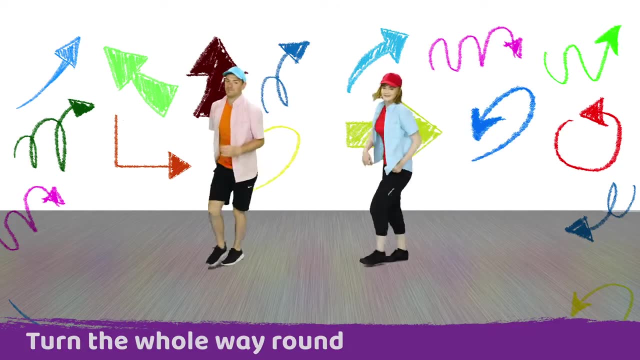 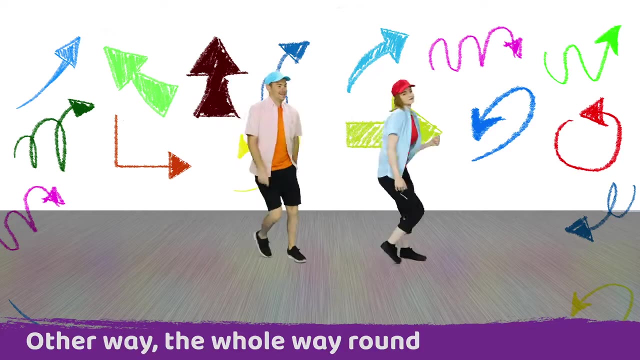 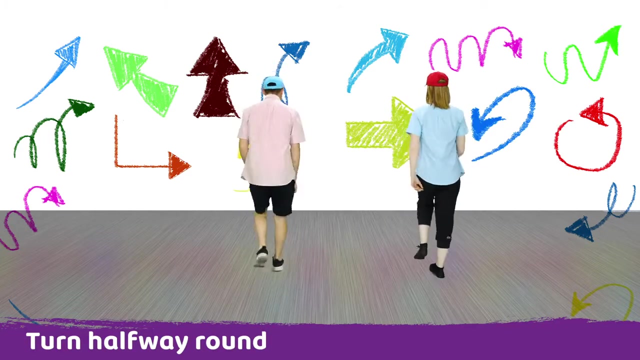 I can go top, I can go middle, I can go bottom, and again I can turn the whole way round. so I am back where I started. Other way, the whole way round. so I am back where I started. I can turn halfway round. so I am looking to the back. 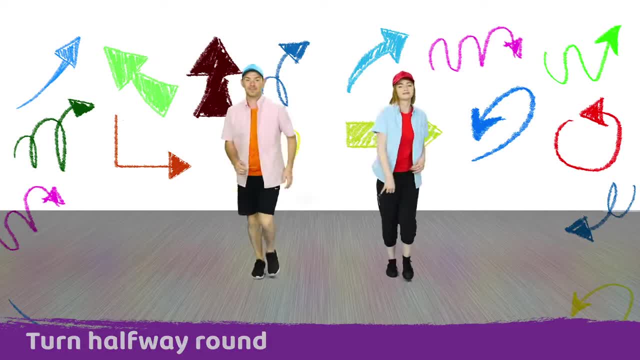 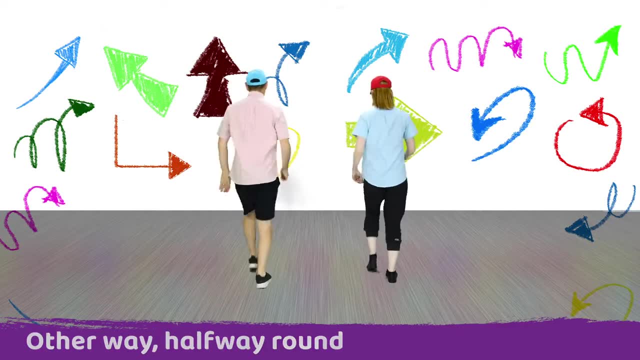 I can turn halfway round, so I am back where I started. The other way, I can turn just a quarter, so I am looking to the side. I can turn just a quarter, so I am back where I started. I can turn just a quarter, so I am looking to the side. 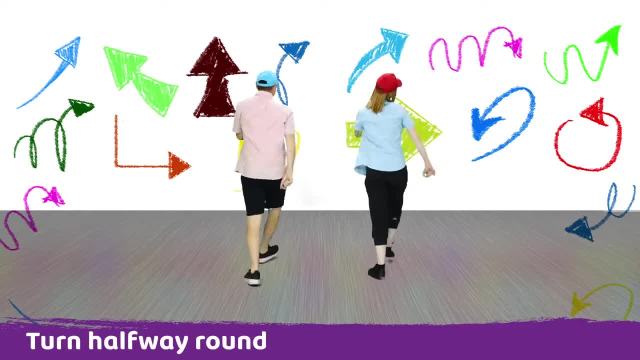 I can turn just a quarter, so I am back where I started. I can turn just a quarter, so I am looking to the side. I can turn just a quarter, so I am back where I started. I can turn just a quarter, so I am looking to the side. 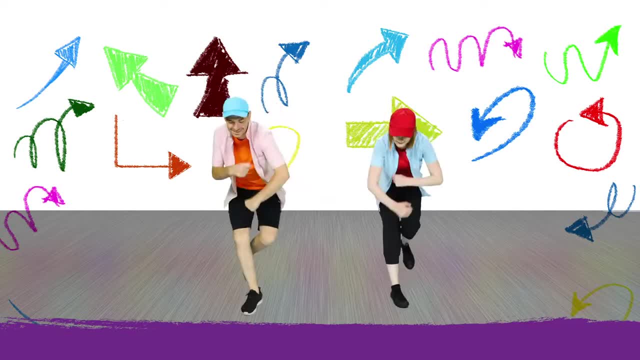 I can turn just a quarter, so I am back where I started. I can turn just a quarter, so I am looking to the side. I can turn just a quarter, so I am back where I started. I can turn just a quarter, so I am looking to the side. 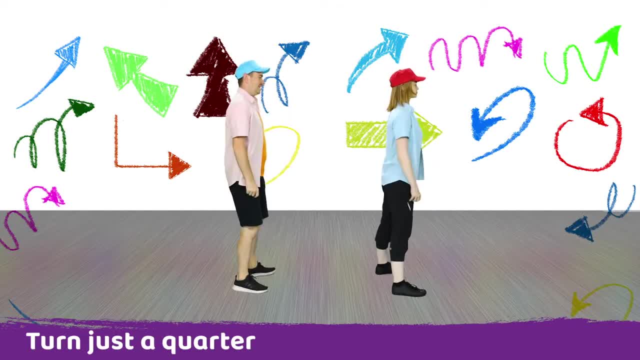 I can turn just a quarter, so I am back where I started. I can turn just a quarter, so I am looking to the side. I can turn just a quarter, so I am back where I started. I can turn just a quarter, so I am looking to the side. 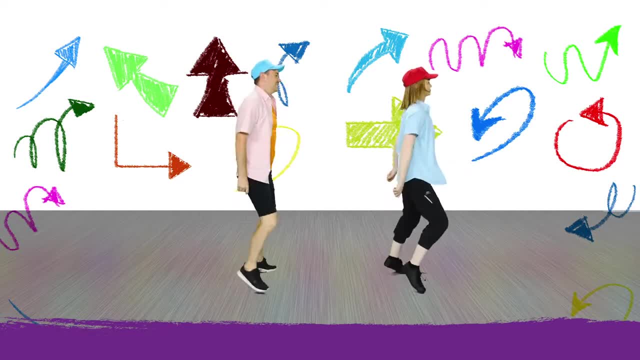 I can turn just a quarter, so I am back where I started. I can turn just a quarter, so I am looking to the side. I can turn just a quarter, so I am back where I started. I can turn just a quarter, so I am looking to the side. 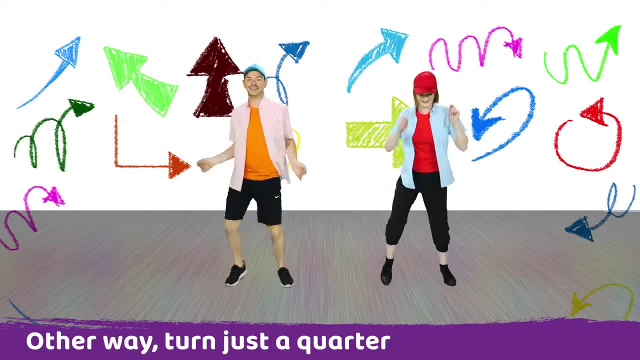 I can turn just a quarter, so I am back where I started. I can turn just a quarter, so I am looking to the side. I can turn just a quarter, so I am back where I started. I can turn just a quarter, so I am looking to the side. 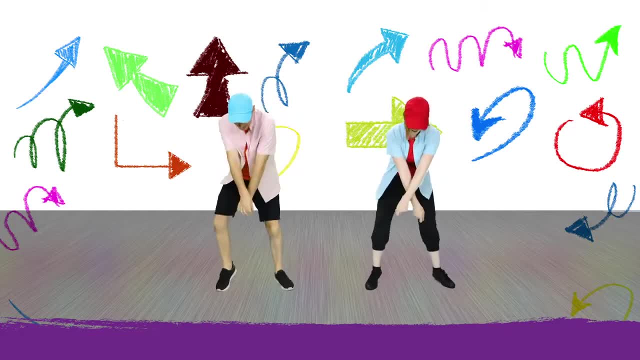 I can turn just a quarter, so I am back where I started. I can turn just a quarter, so I am looking to the side. I can turn just a quarter, so I am back where I started. I can turn just a quarter, so I am looking to the side. 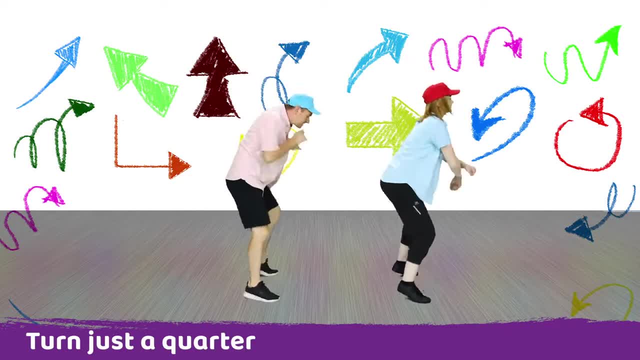 I can turn just a quarter, so I am back where I started. I can turn just a quarter, so I am looking to the side. I can turn just a quarter, so I am back where I started. I can turn just a quarter, so I am looking to the side. 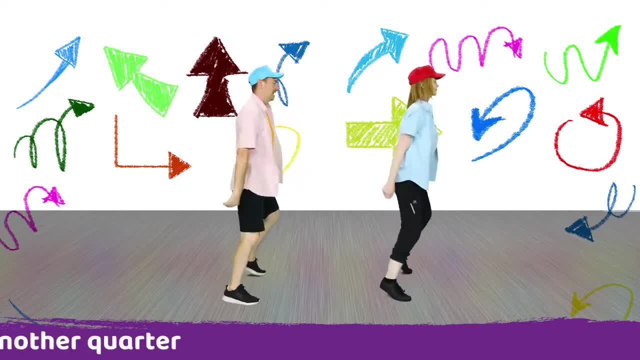 I can turn just a quarter, so I am back where I started. I can turn just a quarter, so I am looking to the side. I can turn just a quarter, so I am back where I started. I can turn just a quarter, so I am back where I started. 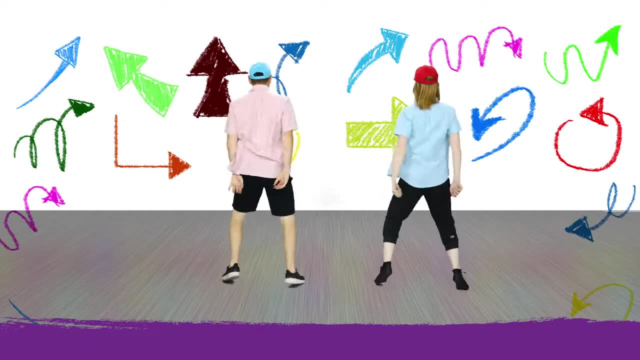 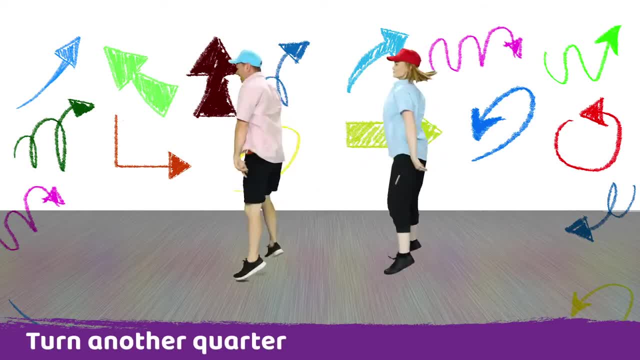 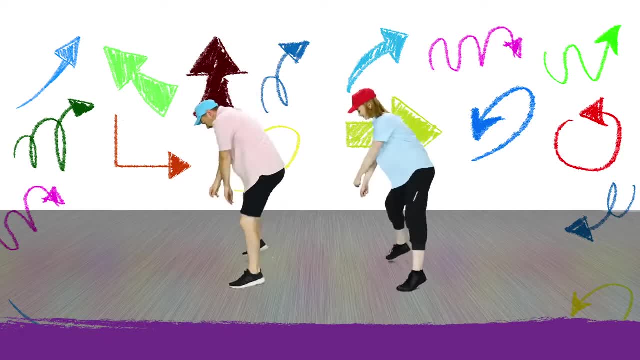 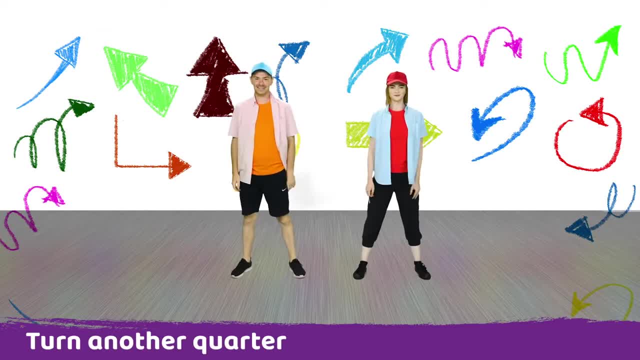 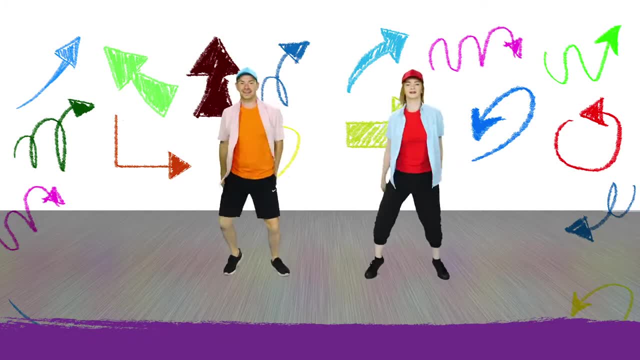 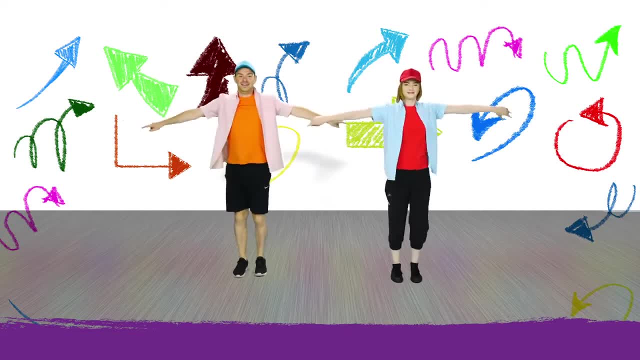 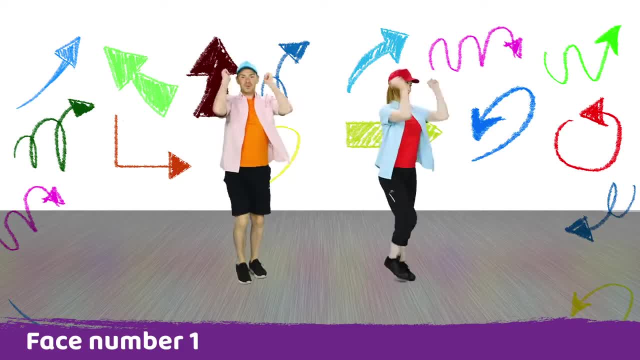 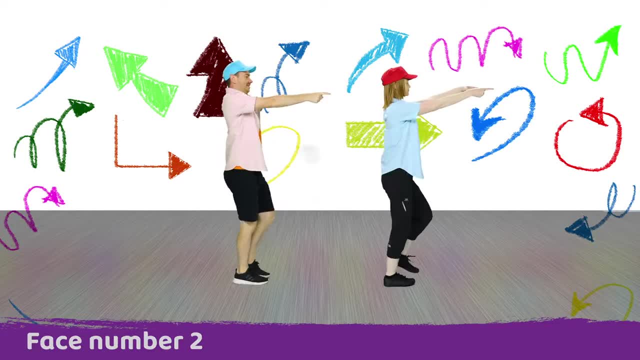 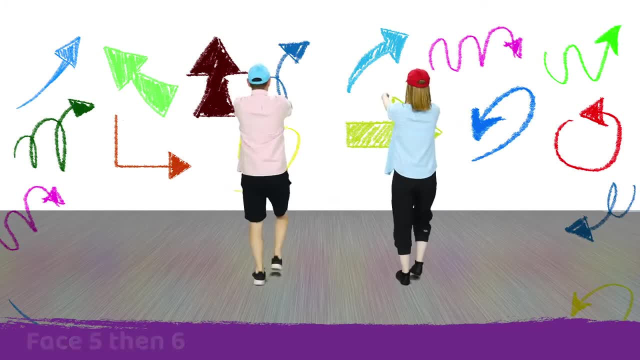 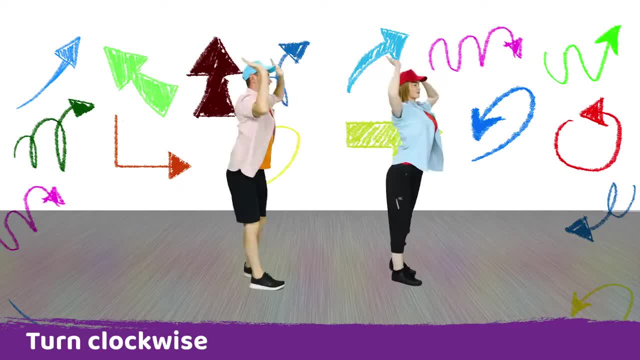 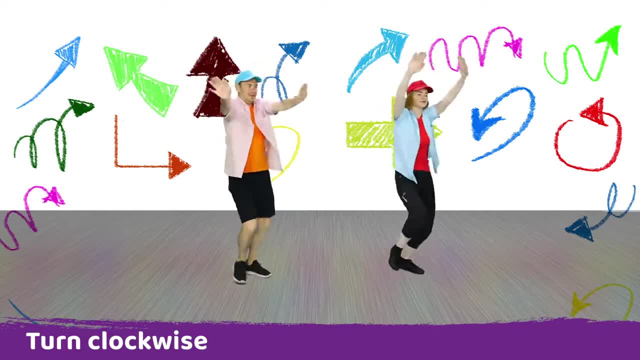 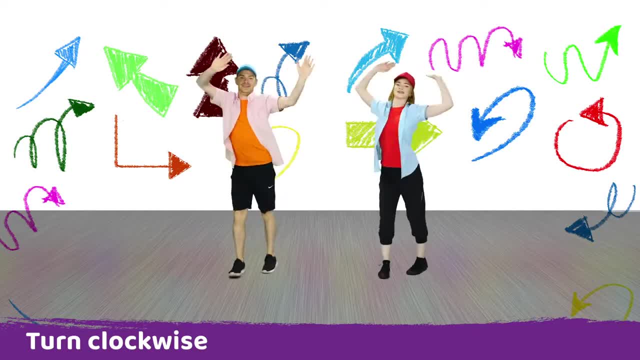 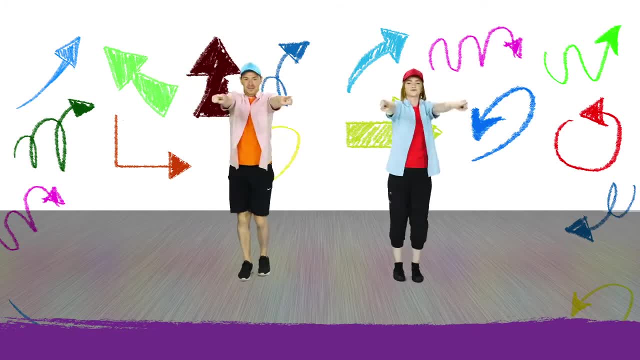 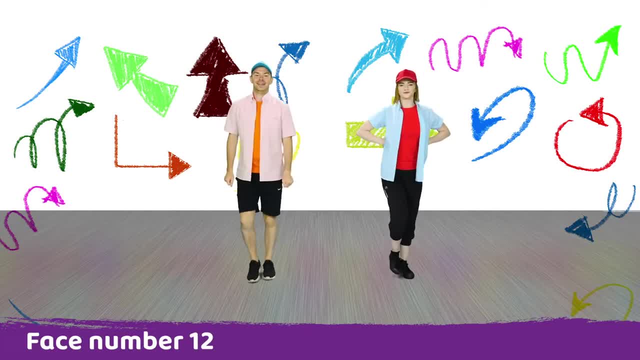 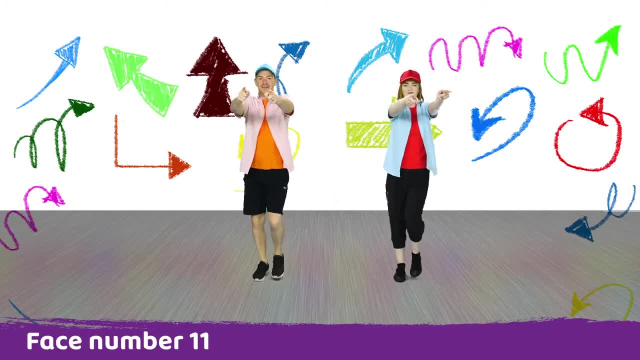 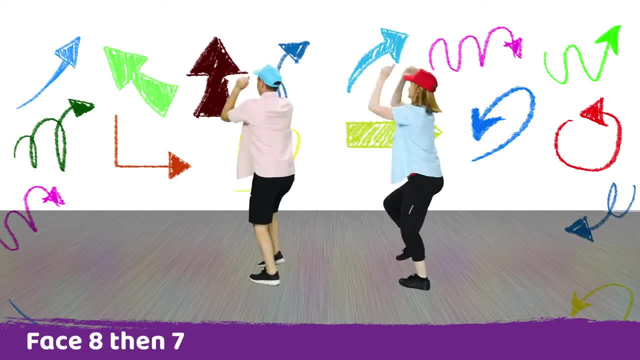 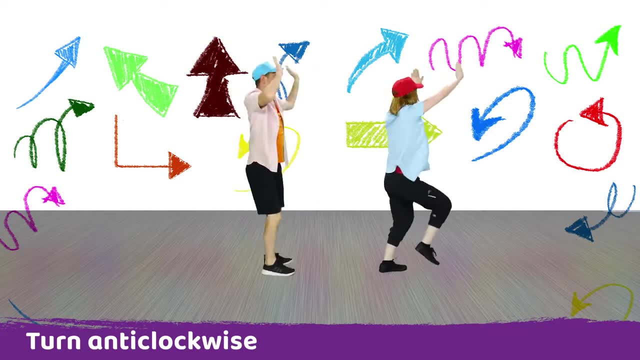 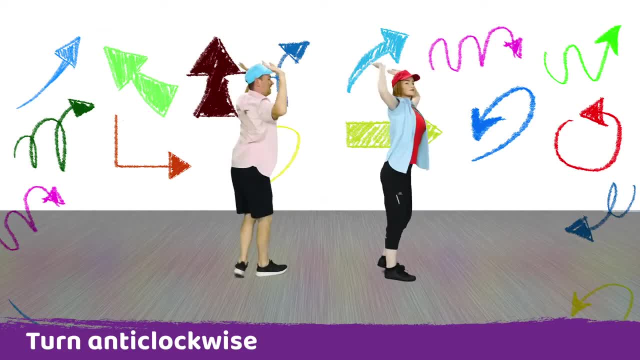 I'm counting backwards. turn anti-clockwise. 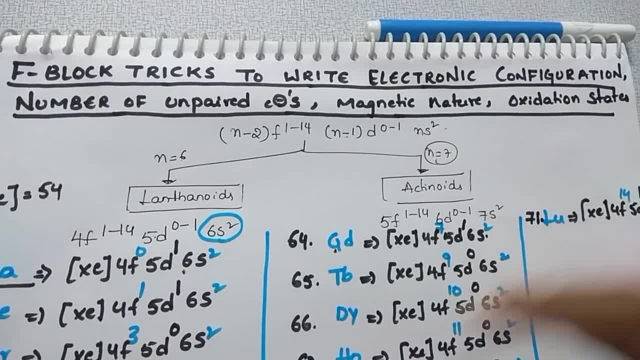 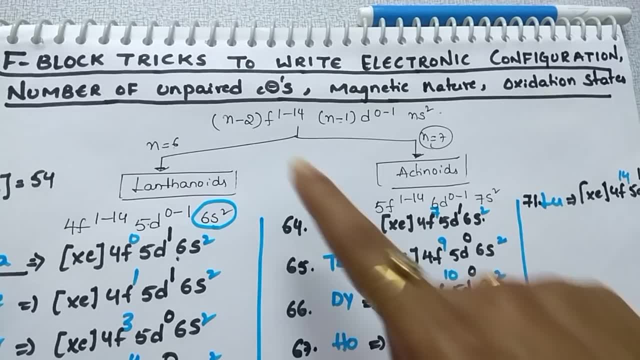 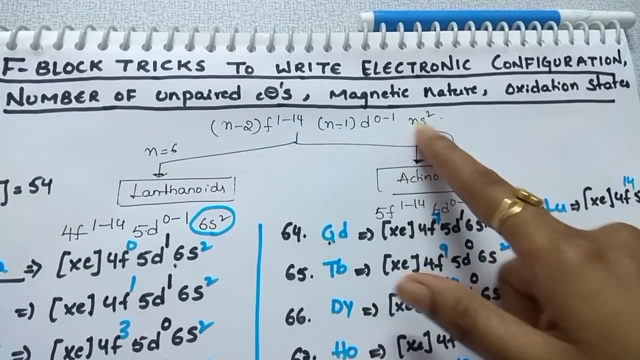 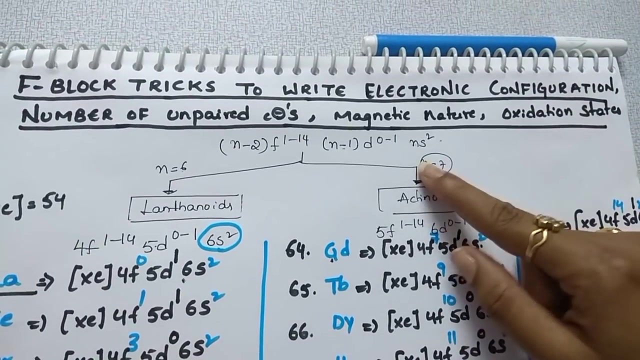 Hi students. in my previous video I discussed about lanthanets. In this session I am going to discuss about the actinets. The general electronic configuration of F block elements is N-2, F1 to 14, N-1, D0 to 1, NS2.. Here N value- if it is 7 means for actinets N value. 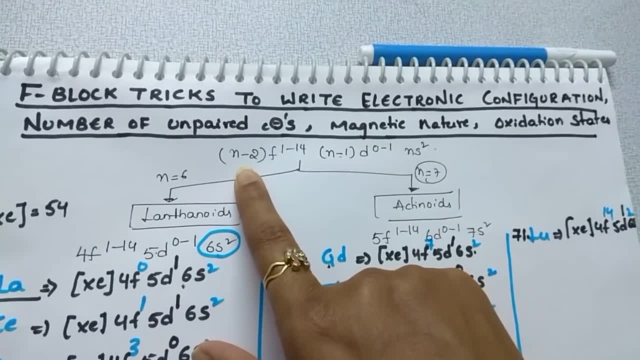 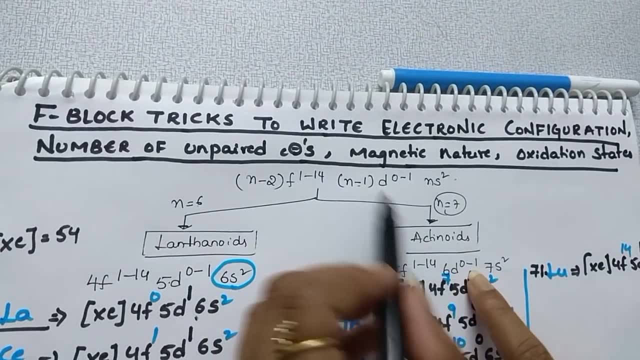 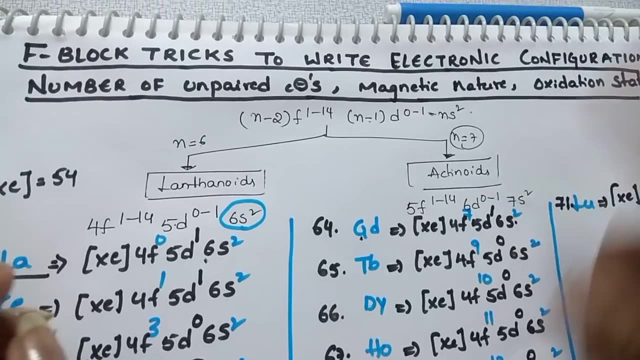 is 7.. Substitute the value of 7 in this formula, then we get 7-2. that is, 5F, 1 to 14, 7-1, 6D, 0 to 1 and 7S2.. This is the general configuration of actinets. So what is the general configuration? 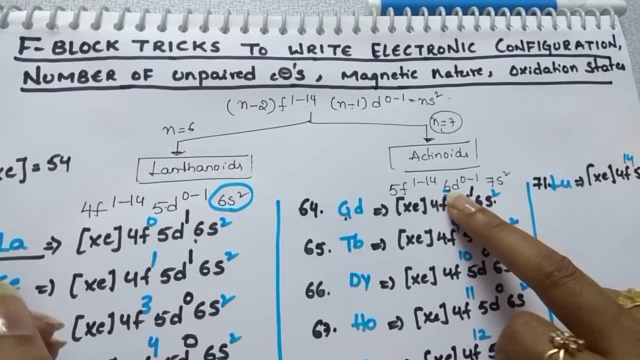 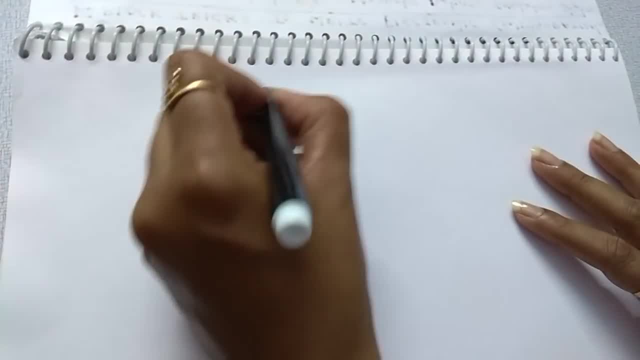 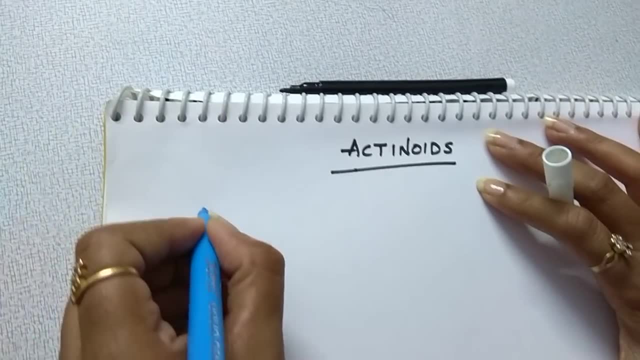 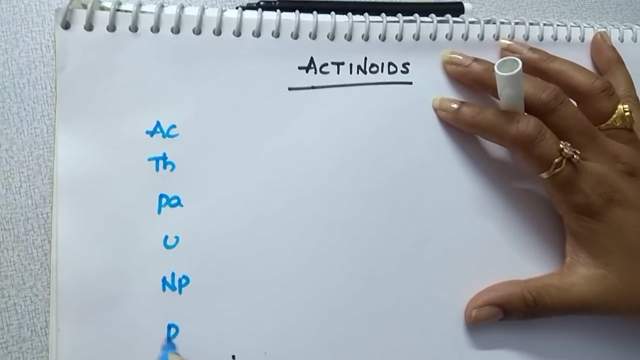 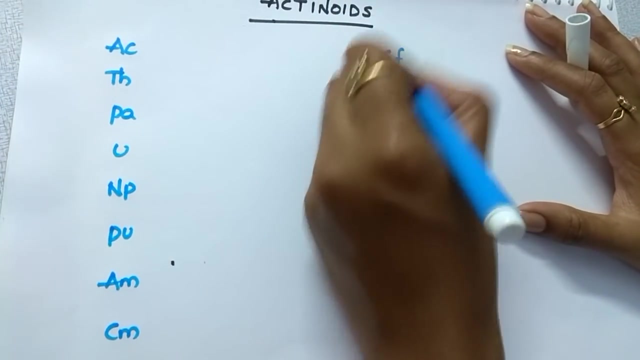 for actinets: students 5F 1 to 14, 6D 0 to 1, 7S2.. Now let us see the elements of actinets. Let us see that, Ok, Ok. 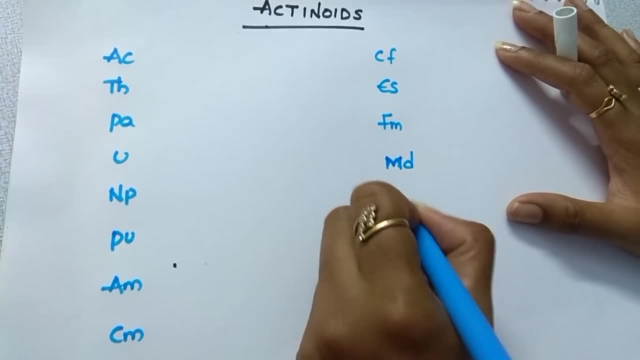 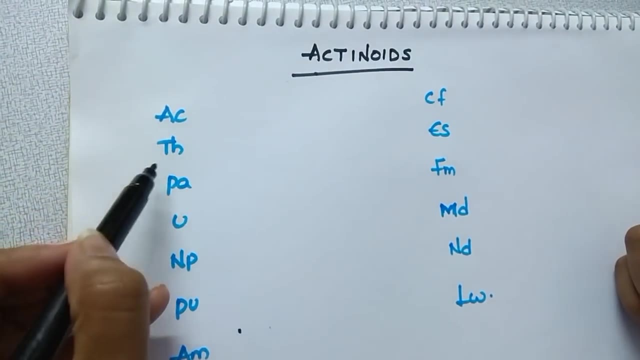 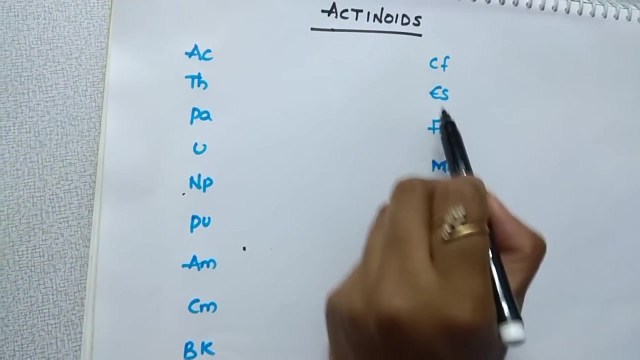